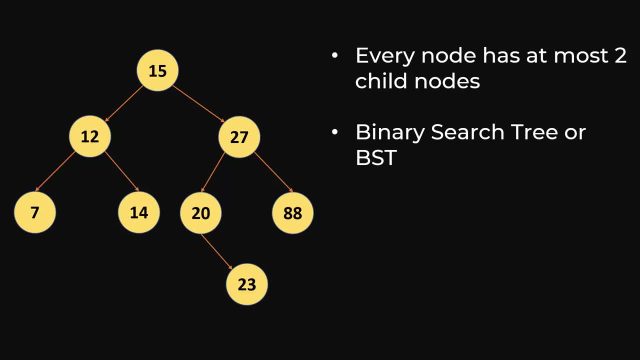 a regular tree with a constraint that it has at most two child nodes. here. this node 12 has two child nodes 7 and 14. 20 has only one node 25, which is 23, but which is okay, the maximum number of on child nodes that a particular node 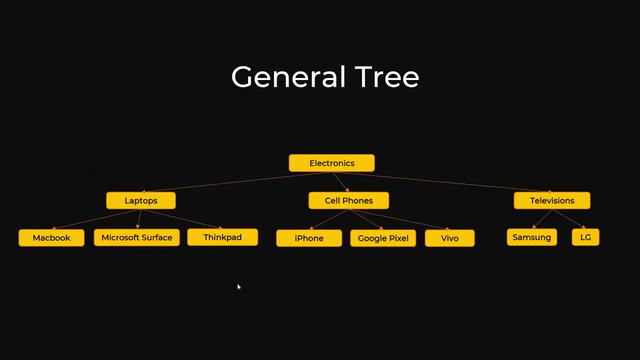 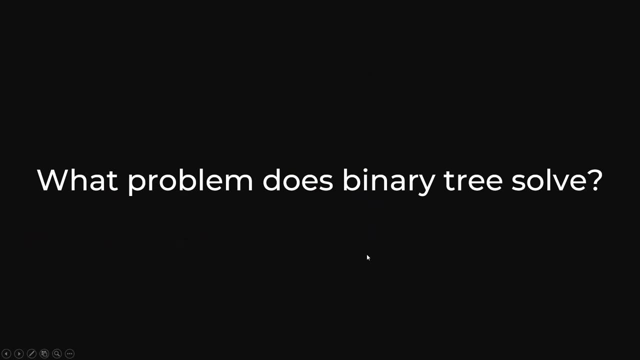 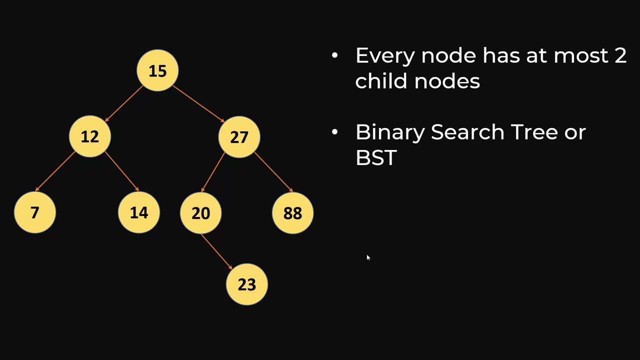 can have is two. if you look at our example of a electronics product tree here, see, cell phone had three nodes. so this is not a binary tree. binary tree is this at max two nodes. now binary search tree is special case of binary tree where the elements have some kind of order. here 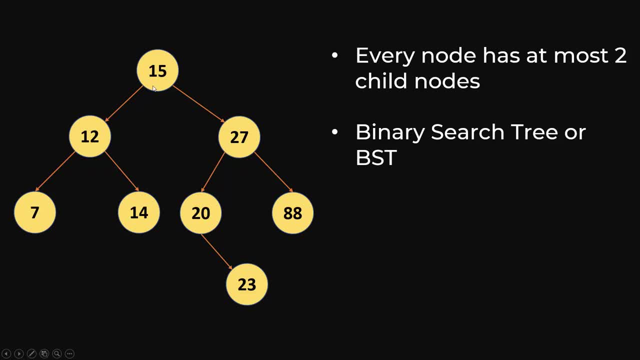 the order is: all the nodes on the left hand side of this particular node has value less than this particular node, so 15. if you look at this whole left tree, all the element values are less than 15 and on the right hand side the values are greater than 15 and that applies to every node. 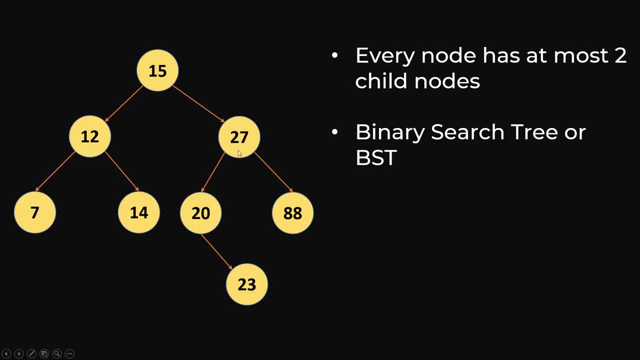 if you look at any node, let's say this: this node 27, on the left hand side, you have values less than 27, which is 20, and 23. right hand side, you have values greater than 27, which is 88. another property is: elements are not duplicated. so if you try to insert 27 again in this tree, it will. 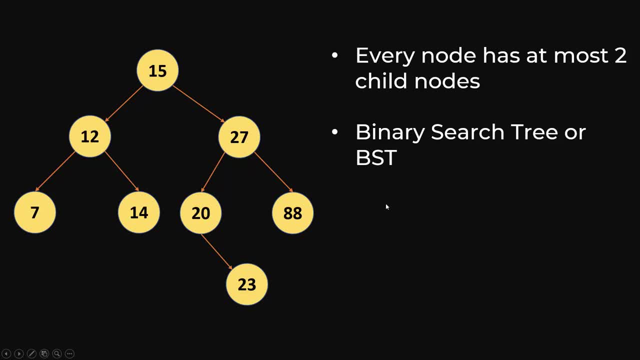 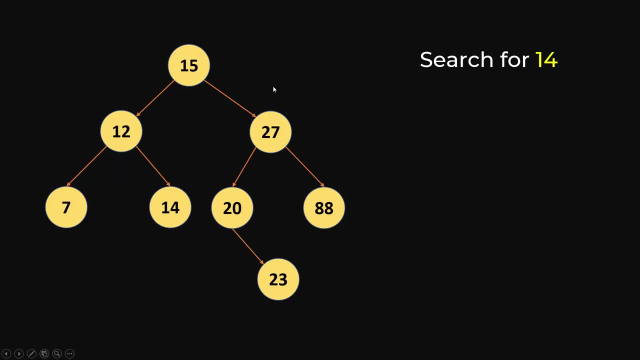 not insert a duplicate. the elements are always unique. now, in this tree, if you want to search for number 14, what you can do is you can start with the root node 15, and then you can see if the value that you are searching for is less than or greater than. 14 is less than 15. 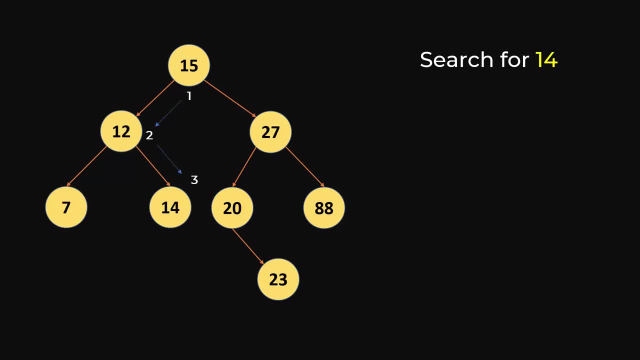 hence you are sure that it will be on a left subtree. so then you go here. you find 12. now 14 is greater than 12, hence you know it has to be on a right hand side. this way what you're doing is in search operation, which is very common in computer application whenever you are writing. 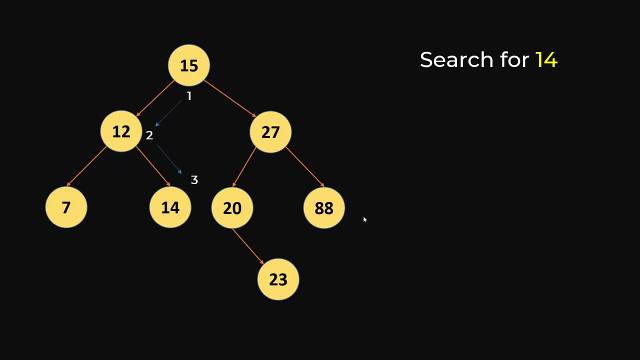 software. uh, searching through a list of elements is a very, very common operation and you want to make sure you do that search in an efficient way. if I had stored all these numbers in a single list, then finding element or searching an element might be linear complexity, because if you search, 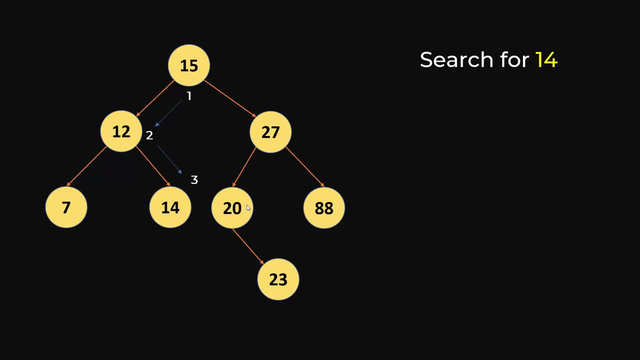 elements one by one, then your complexity will be order of n. but if you search this way, then what? every time you are reducing your search space by half. for example here, when you decided that 14 will be in a left hand side tree, you eliminated searching right tree, so you eliminated you. 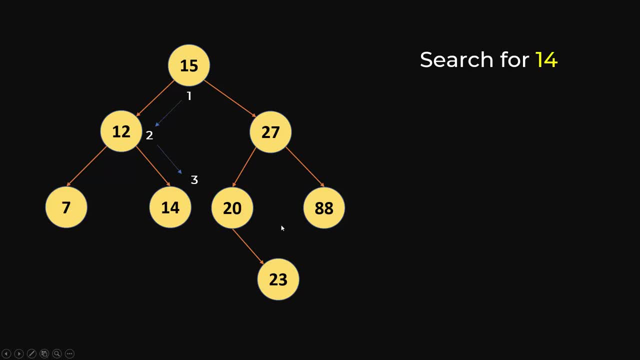 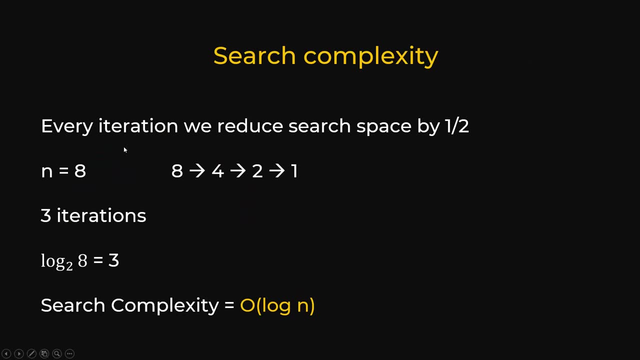 eliminated these four elements. uh, right on a first go. so, thinking about search complexity, since we, let's say you have, our number of nodes in a tree is eight, when you search for an element, when you make a decision, whether the element is in a left tree or right tree, you are reducing the space by 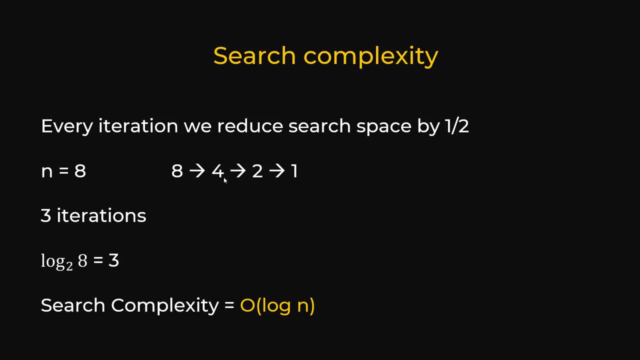 half. so now your space is four. then in that tree, when you further search, you make the search space by two one. so for, if the total number of nodes in your tree is eight, you can search an element in three iterations. and three now, compared to eight, is nothing but a log to the base two. hence the search complexity in binary. 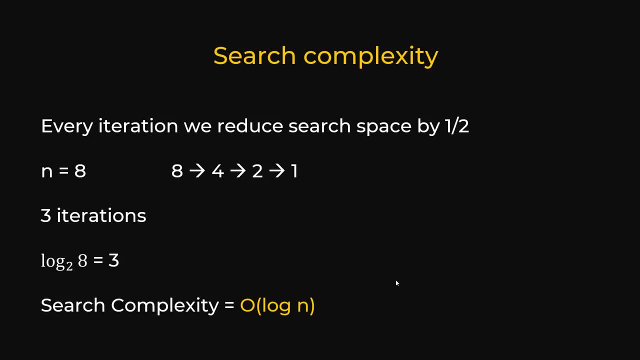 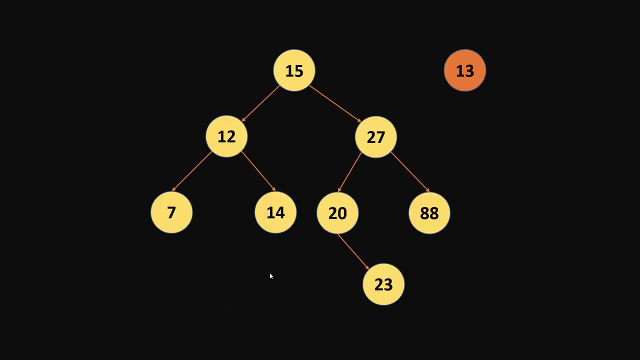 search tree is order of log n, which is very efficient operation, like, if you think about it, for eight you achieved your search result in only three iteration. if you had done linear search you might have to do eight iterations. now let's talk about inserting an element. let's say you want to 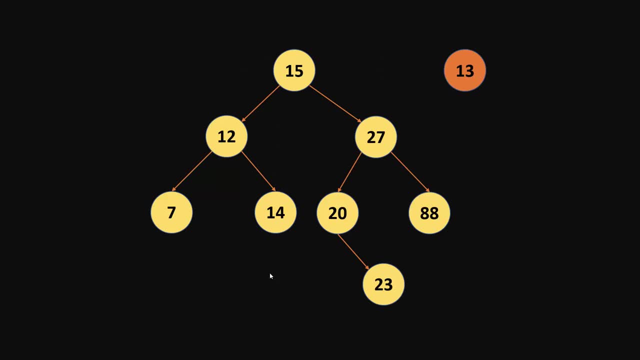 insert number 13 in this binary search tree. what you can do is first compare it with 15. you know that 13 is less than 15, hence you want to put it in a left subtree, so you will come here. now you realize that 13 is greater than 12, so it will. 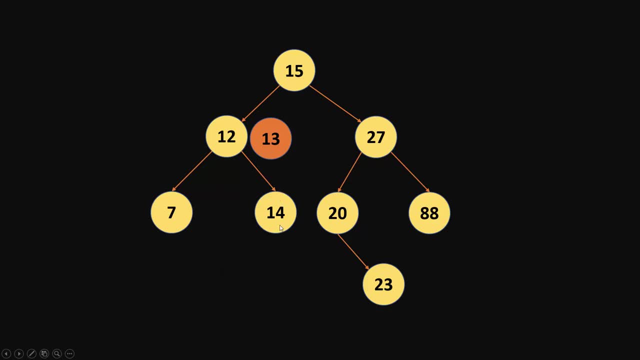 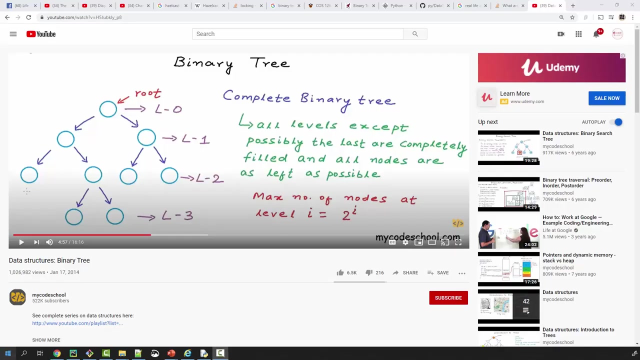 go in a right subtree. then you come to 14 here and then 13 is less than 14, so you insert it in a left subtree of 14.. here the insertion complexity is also order of log n. there are certain terms associated with binary tree in general, such as: 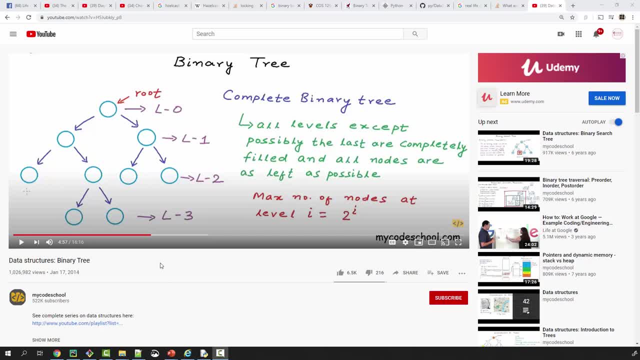 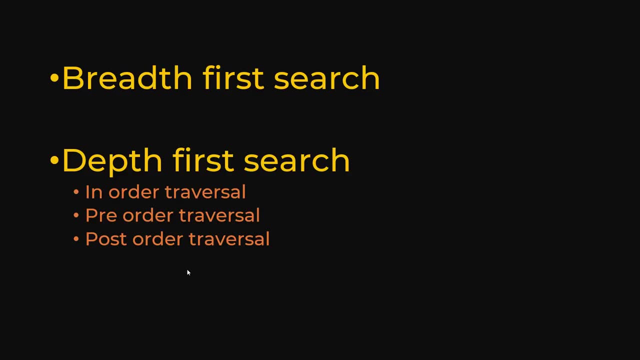 level, depth, number of elements, and there is this great video which will clear all your terms, so I highly recommend watching this video. I'm going to provide a link of this video in a video description below if you want to search through the binary search tree, there are two approaches. 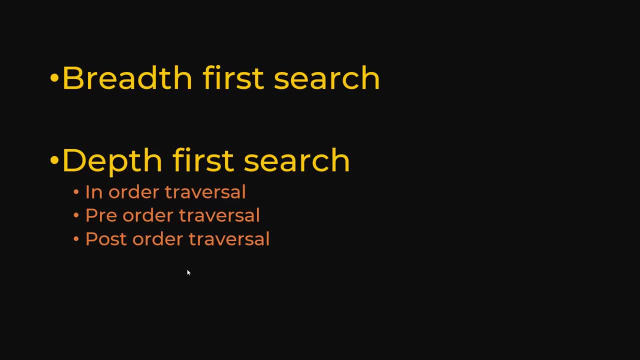 you can take. one is breadth first search and the second is depth first search. these are also called traversal techniques, which means how do you traverse your binary tree to find the element that you're looking for? in this coding tutorial, we are going to cover in order, traversal, which is 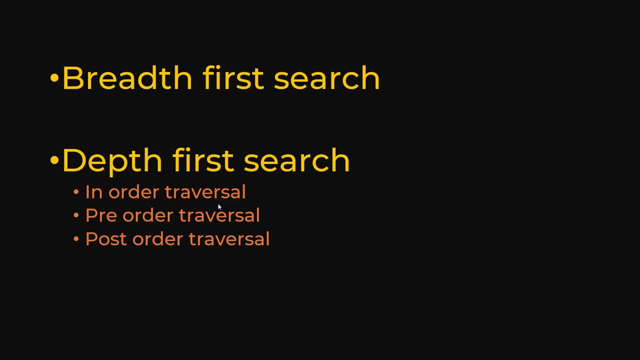 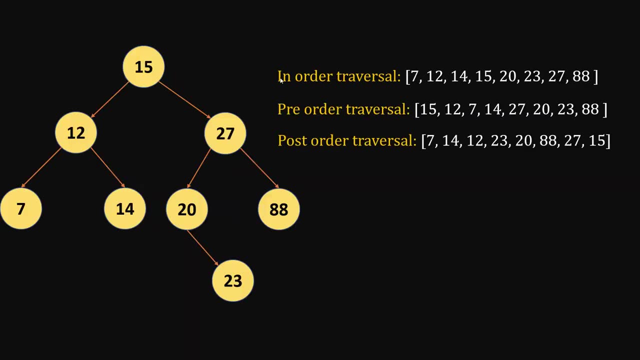 a depth first search traversal technique. so let's go over this depth first search traversal techniques a little bit. so let's say, if you have a tree like this in the in order traversal, what you do is, you see, when you say in order or pre-order or post-order, you are referring to your base node. so here the base node. 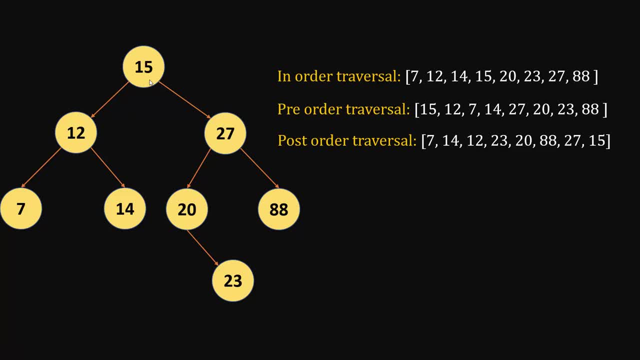 is 15.. when you are doing in order traversal you try to make sure this 15 node is in the order, which means you first visit your left subtree, then this particular node and then right subtree in in pre-order traversal. actually you for you visit your root node first, then left subtree and then right subtree and in the post order you visit your. 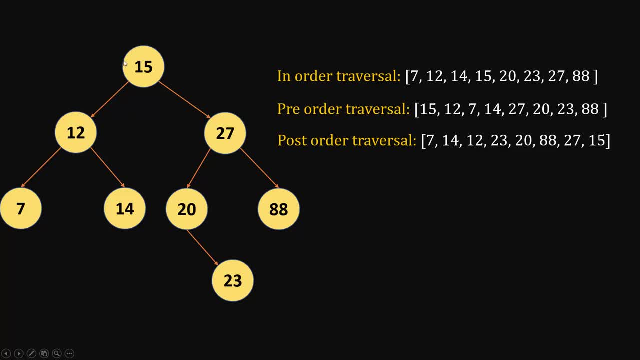 left subtree, then right subtree and then your root node. so for example, in in order traversal: okay, what you do is first you take left subtree, so when you are traversing this particular node 15, you come to left subtree. now, how do you traverse left subtree? well, you apply recursive technique here. so here: 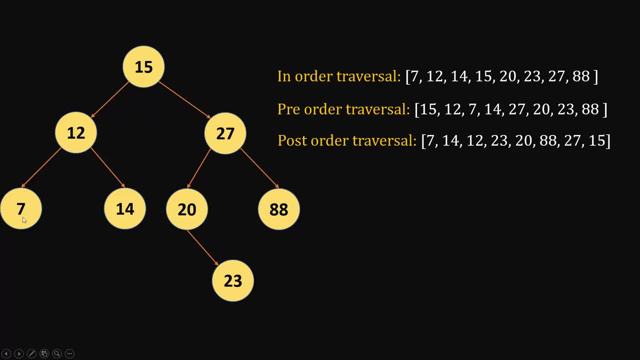 again. you apply the same rule for 12. the left subtree is 7, so first you use this 7, then you use it 12, then use it 14.. so you get 7, 12, 14.. now your left subtree is done, so you visit root node. 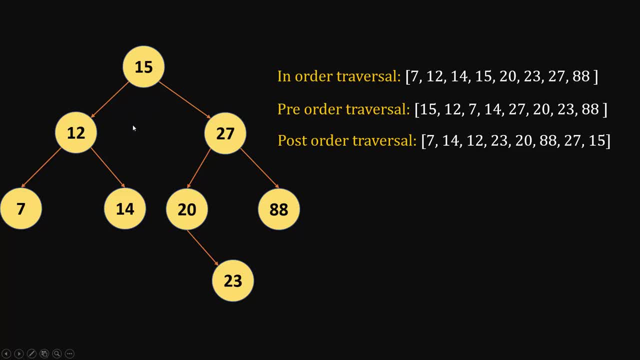 which is 15. so you see 15 here. then you visit right subtree. okay, right subtree is these four elements. there also, you apply recursion and you first visit left subtree of 27, which will be 20, and if you recurs, if you traverse that, you will get 20 and 23, then 27 and then 20 and then 88 in pre-order. 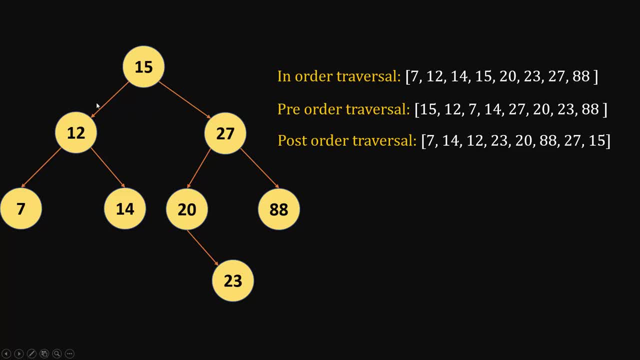 you first visit the root node, which is 15, then left and right subtree. uh, remember, we always visit left subtree first and then right subtree, then after right subtree. then again you see 20 and 23, then 87 in pre-order. you can begin work on them alternately. 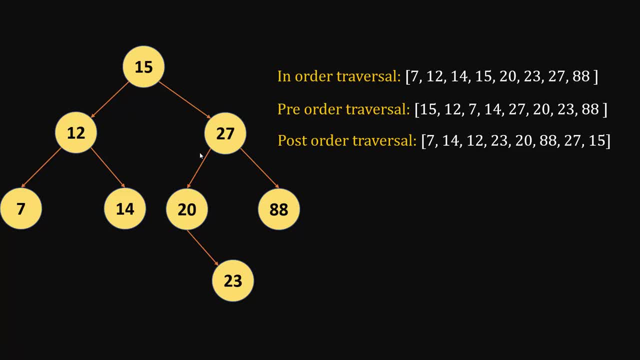 tree. we never do right or right first and left after that in any of these techniques, so that's an easy way to remember left and right. they're always in sequence: left comes first, right comes second. now pre-order- post order in order is decided by where do you put your root node in? 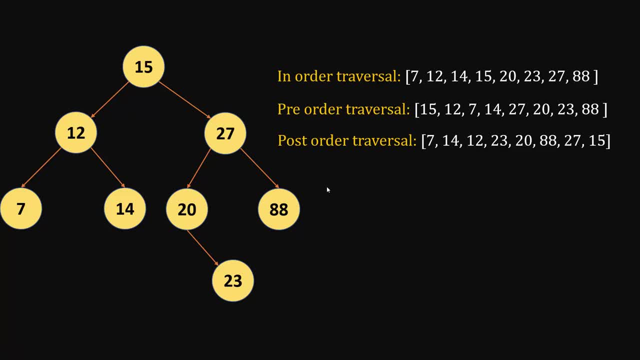 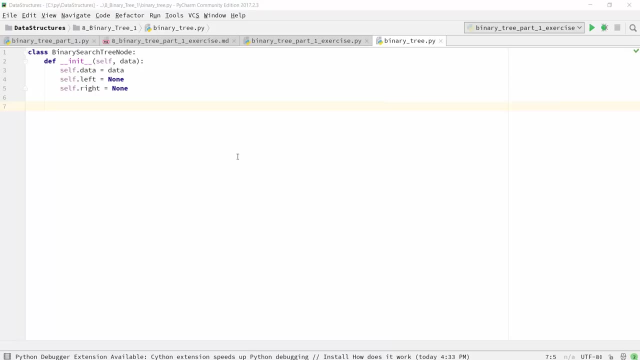 between your left tree and right tree. if you put your root node in between left and right tree, it's called in order. if you put your root node before left and right sub tree is called pre-order. so this is pretty easy to remember. now let's uh get into coding. here i have defined binary search tree. 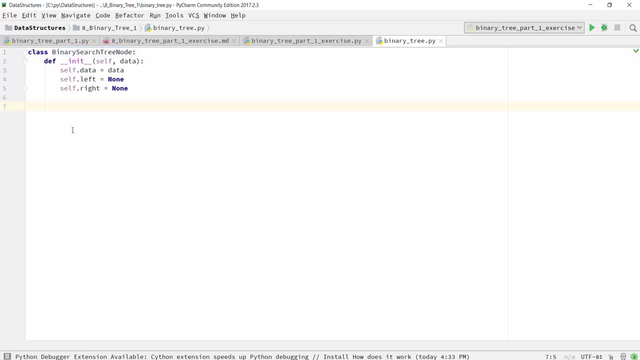 node class. remember we are implementing a binary search tree, so there is a general tree which can where a node can have any number of elements. binary tree will have at max two elements and binary search tree is a binary tree with a specific order, where left search tree has all the elements which are 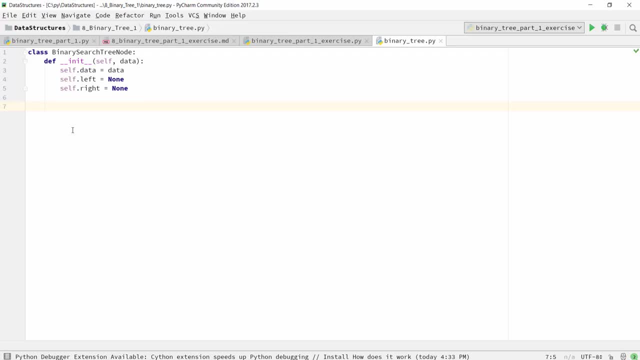 less than the current node and the right hand side has all uh greater elements. so when you add a method called call, add child here, what i want to do is here, uh, i, i have this node. okay, it could be a root node, it could be any node in the tree, and whenever i want to add a child with a value, 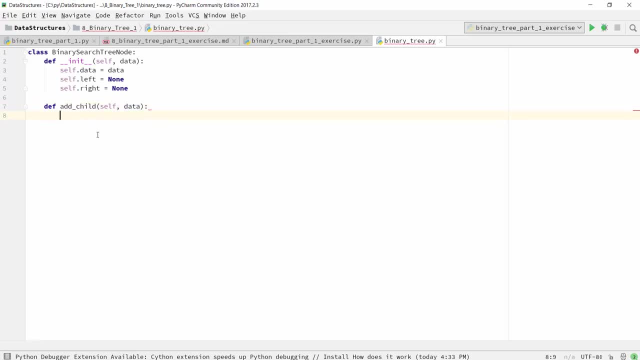 data. i need to check the value first. so what i need to check is if data is equal to selfdata, which means the data that i am adding a that value already exists. see, if the value already exists, then you don't need to add anything, because binary search tree cannot have duplicate elements. so 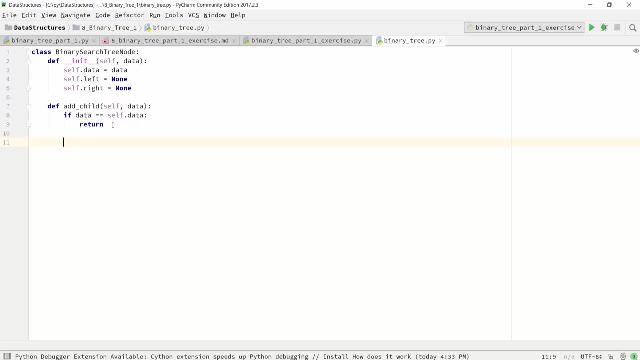 here you just simply return. but let's say that is not the case and the data that you are adding is less than, uh, the value of current node. what this means is: here we will have to add this value, which means data in left subtree, okay, and if the value is greater than, 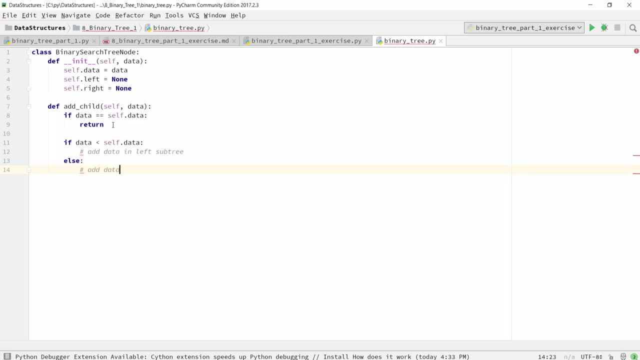 then add data in right subtree, correct, okay. now let's write code to add it in a left subtree. so in a left subtree. first you need to check if your left element has some value, which means you are not a leaf node, okay, uh, if you are in else case, then it means that your left 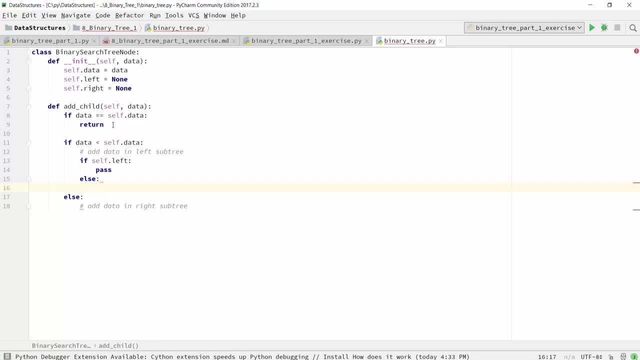 node is empty, okay, and if left node is empty, then it's very simple. you can just say: selfleft is equal to binary search tree node of value data. so tree is a recursive data structure. hence you can just create a tree node and that node will have a value, is equal to data. so if you 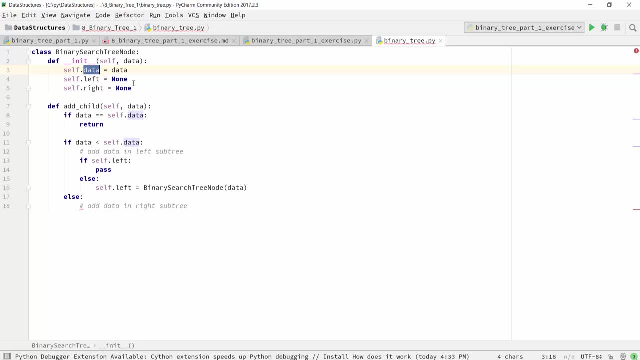 look at the constructor: data goes into selfdata and then left and right child would be none. and you created that node and assigned it to selfleft. but let's say selfleft already has some tree, some value. then what you will do is you will say selfleft. 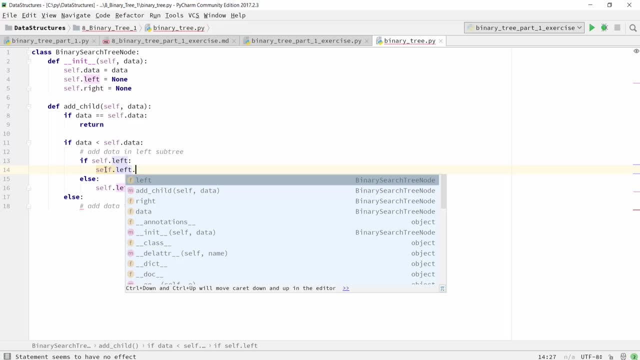 dot. think about it. what will you do here? well, you will recursively call add child method with value data, because dot left itself is another small sub tree which will have add child value. so you can call that method with data and it will go into recursion. it will go. 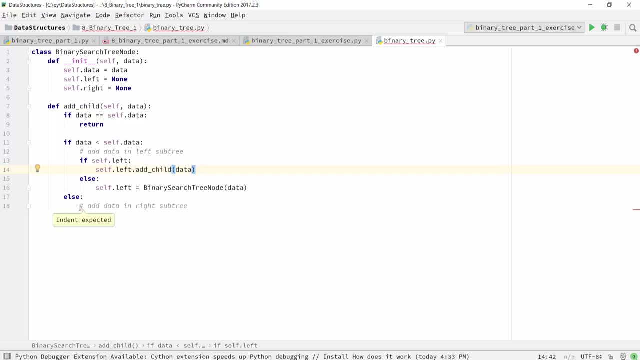 come here and you know it will just work out. similarly, you can add code for your right sub tree. it will be very similar code. okay, and once you have done this, now what we are going to do is: now I will implement in order traversal method, because using that method, I can print all the elements in my tree. okay, so I 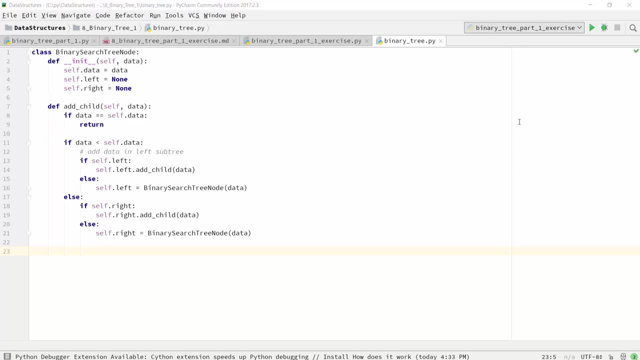 will define this method called in order traversal, and here this method will return a list of elements in your binary tree in a specific order. you can see that I have created a list of elements in my tree and now I will call it in order traversal. okay, so let me just call elements as elements. so my 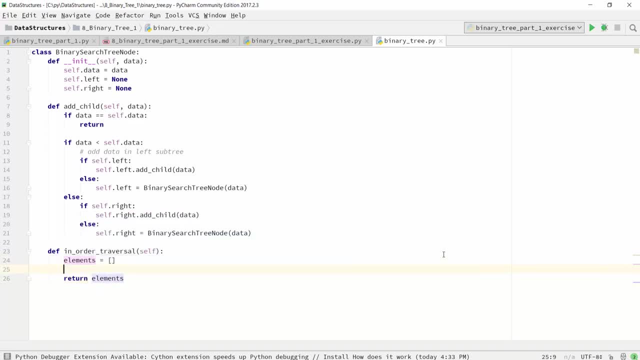 goal here is to return these elements, and here here I want to fill this list with all the elements in a binary search tree in a specific order. now, what is the specific order? in order, traversal means first you are visiting your left sub tree, so you need to check if self dot left meaning. 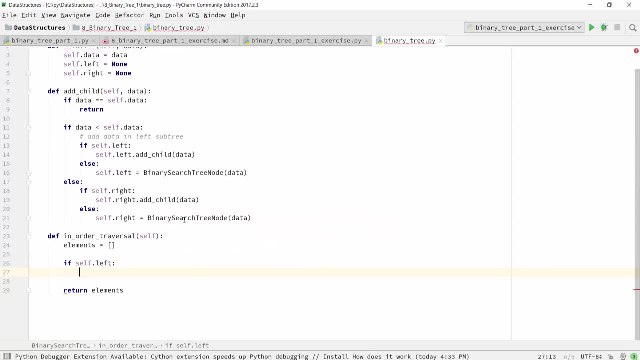 on the left hand side you have some elements. then you can say elements is equal to self dot left dot in order traversal. it will require some thinking to understand this recursive method. when you say elements is equal to elements plus something, this method will return some and it will add that list to this particular list. now here it will call: 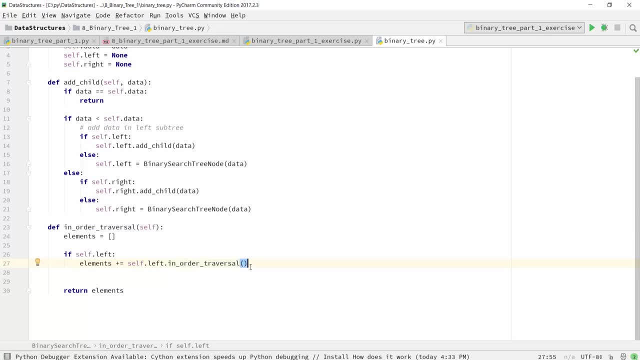 this function recursively, and when does a recursion end? well, we need to write some more code here, so just assume that this method will work. okay, so just leave this for a side. in order, traversal means you visited your left tree, then you visit the base node and then you visit a right tree. so let me write it down to: 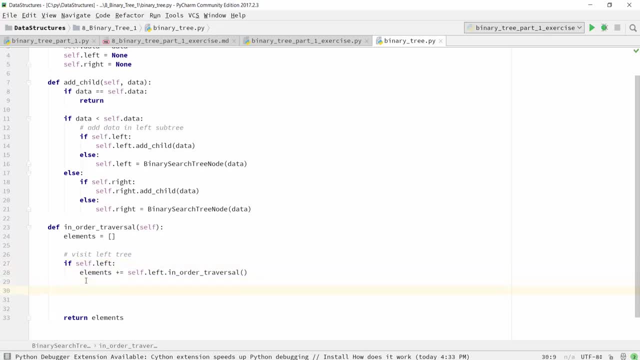 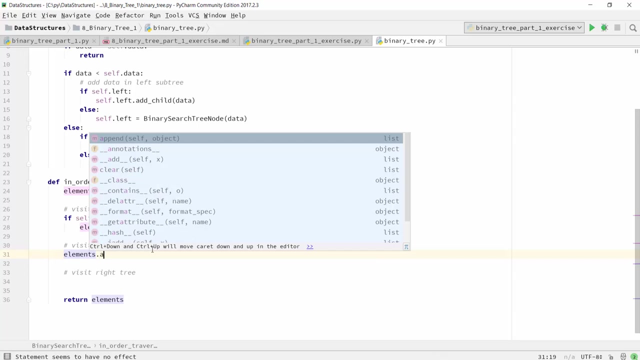 visit left tree first, then visit the base node, which means this particular node, and then visit right tree. okay, so let's visit the base node. so the base node is nothing, but in the elements you append self dot data, which means this particular node. now happens when the data machine cuz, that data machine will. 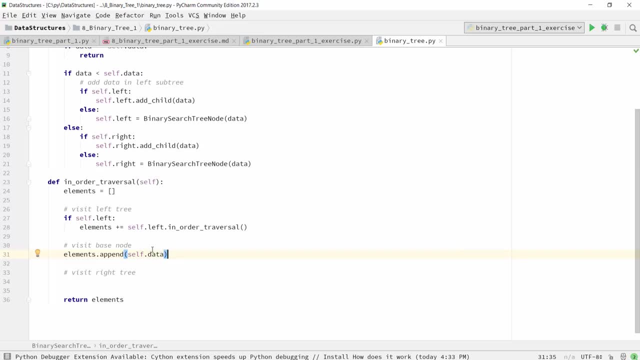 last very long time for the right tree in which one of these data is given. so so let me you make sure the basic node is no. okay, let me make sure need to miss node has a value data and that I want to insert in elements, so I inserted. 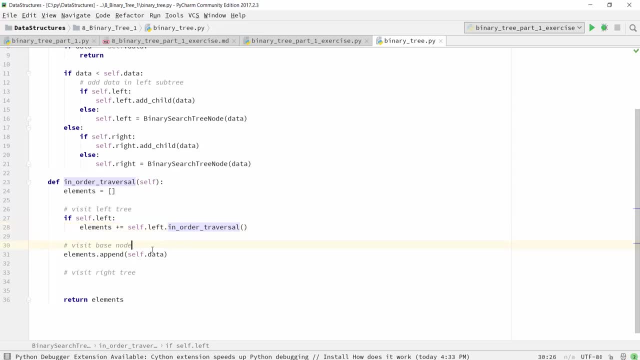 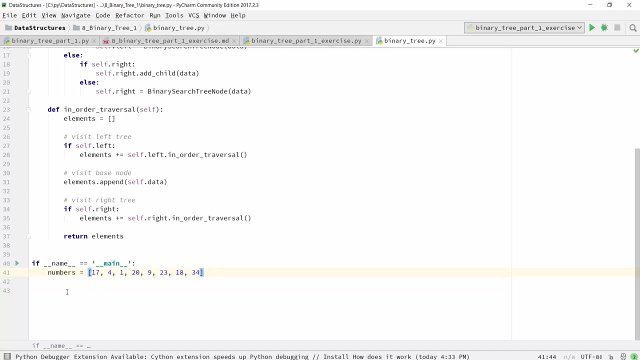 elements from the left subtree, then this particular node, and now I will do same for right subtree. so if self dot right, then elements is equal to elements plus self dot right, dot, in order: traversal. here I have written my main method, where I have these list of numbers and I want to build a tree out of this. okay, so let. 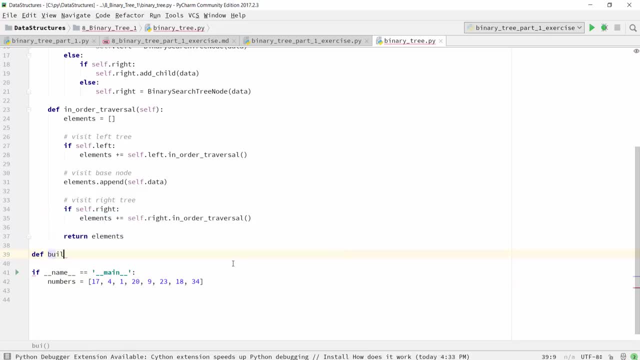 let me write a helper method called build tree and this build tree takes elements as an input and this will build that tree for you. so your root node will be your binary search tree node and let's say you assign the first element here as a root node. 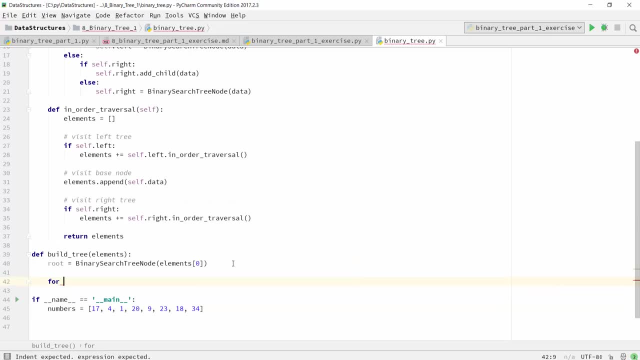 and then you run a for loop on elements which are from which are in range 1 to the length of this elements. okay, so we are going through this list and building the tree, and to build a tree we already added add child method here. so here you can just. 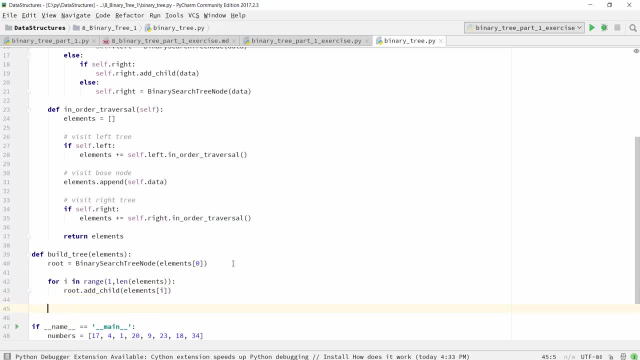 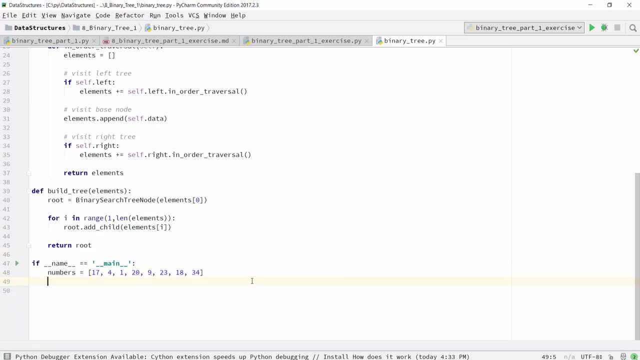 simply say add child and then, once the tree is built, you return this root like this: okay, so here I can now say: numbers tree is equal to build tree with numbers, and once the tree is built, I would like to print it. and the way you print it is by doing this traversal. see if I do in order. 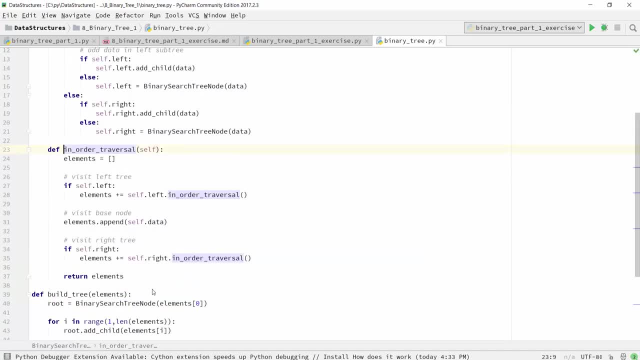 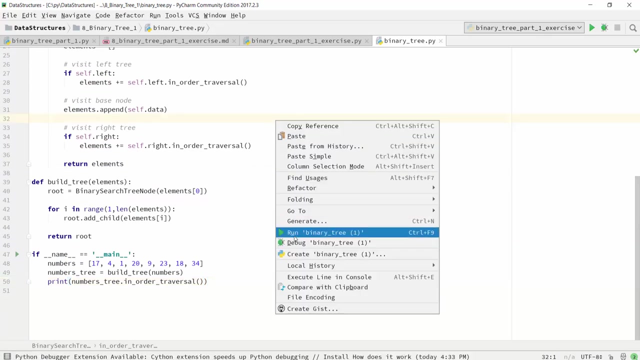 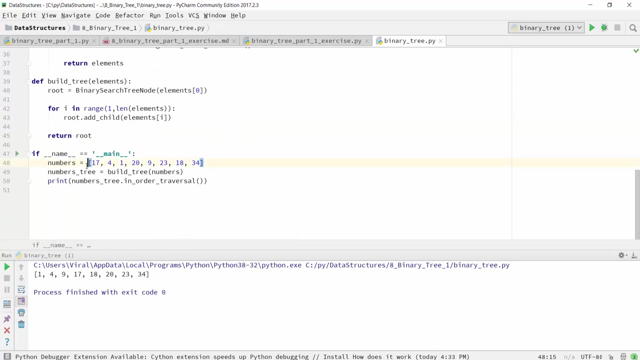 traversal this particular method. if you look at this method, it returns all the elements in the tree in a specific order, in an ascending order. okay, so let's run this code and see how this goes. great, so you realize that when I give this list, it will build a tree and then, when you do in order, traversal it. 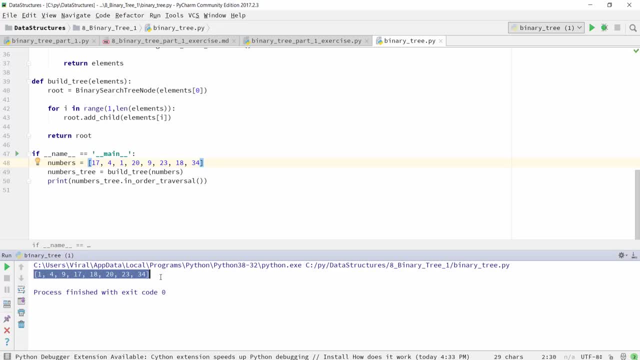 returns a list in a sorted order. so one of the utilities that I have here is a of binary search tree, is to sort the elements in the list. the other utility is, of course, to implement set type of class where the elements are unique. so here, if you give same element, let's say, 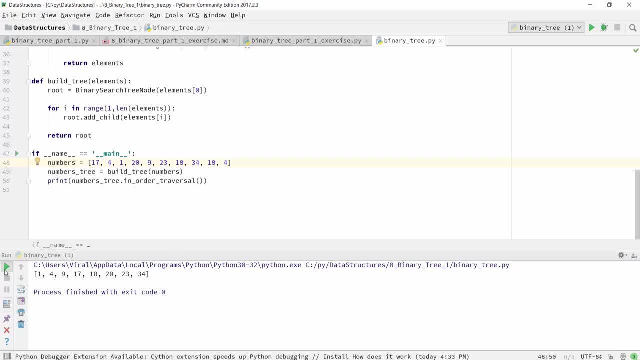 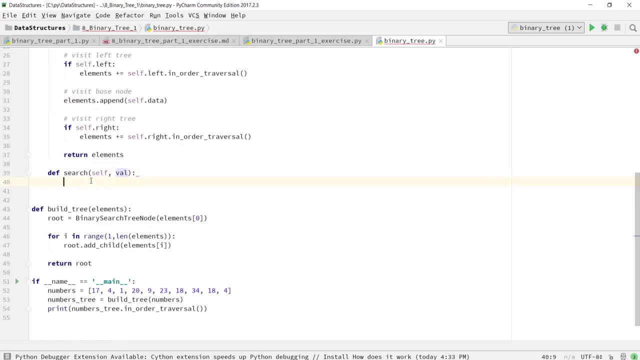 i give 18 and 4, it will remove those duplicates. see: 18 and 4 appeared only once. so to implement set. this can be very useful. now i am going to implement a search method here in my binary search tree class, where you are searching for some value now the first thing, obviously, that you do is: 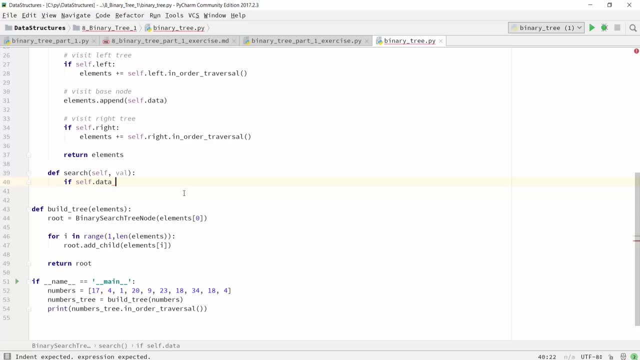 if your yourself dot data is equal to the value that you are searching for, then you are lucky. you can just return true here. but let's say, if the value that you're searching for is less than self dot data, what does this mean? well, this means value might be- it's not guaranteed to be, but it might be in left subtree. 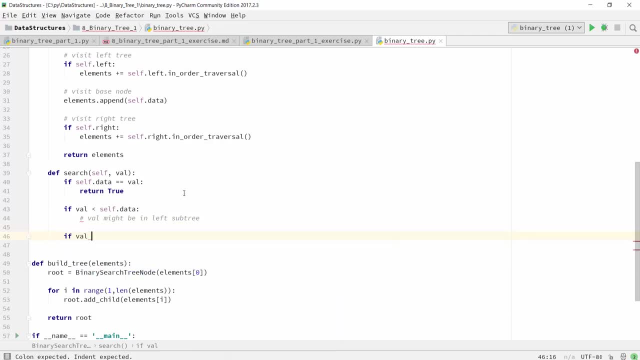 okay. and if value is greater than self dot data, then it means well, might be in right sub tree, okay, so if it is in left subtree, how to implement it? first you check if self dot left in my left subtree. do i have any content? okay, let's say that is yourself. dot left is none. 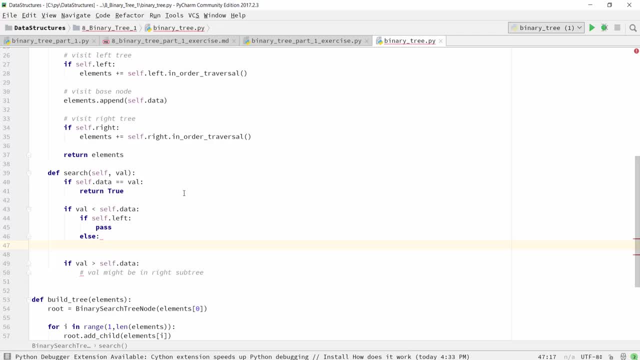 you know you don't have anything, which means you have, you have reached an end and you can safely say return false, which means it's a self dot, which means it whole child happens somewhere, because the eight two set itself doesn't exist in my tree. but what if there is a left subtree? 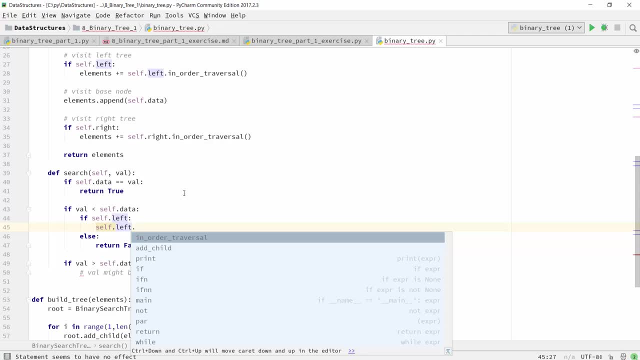 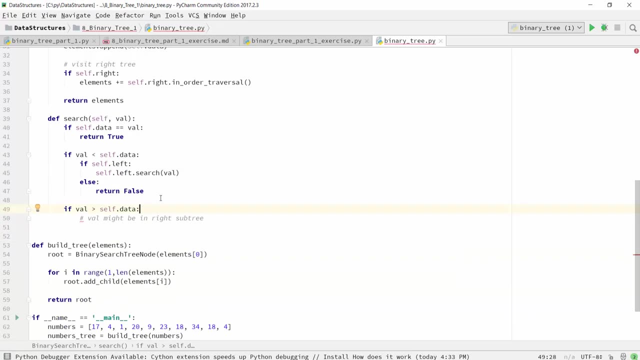 well, in that case you can again call a recursion. you can say: self dot left, now in my left subtree, search for this value. well, okay, so i hope it makes sense. it will do a recursion. it will further go into left subtree and run the same function. see, this search is the same function now in my left subtree. 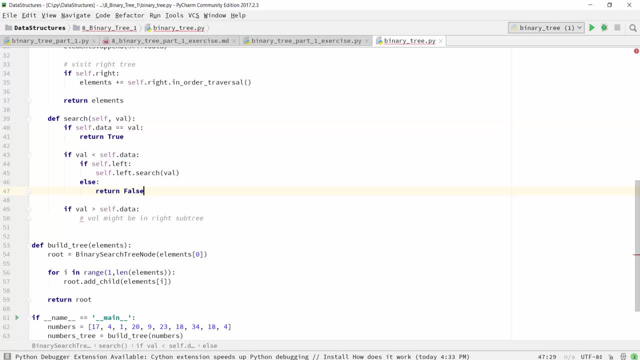 okay, so i hope it makes sense. it will further go into left subtree and run the same function. see this search is the same function that you're calling, and this concept in computer science is called recursion, and you'll do the same thing for your right subtree as well. now let's test this method to see. 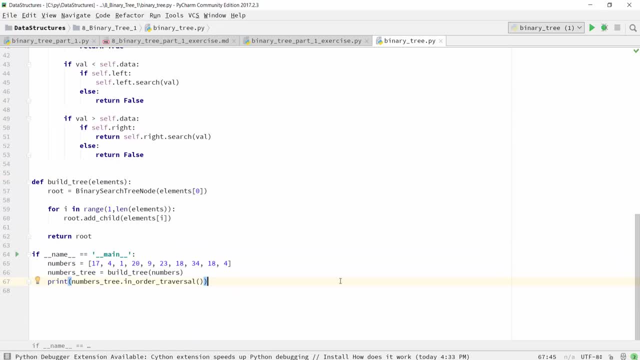 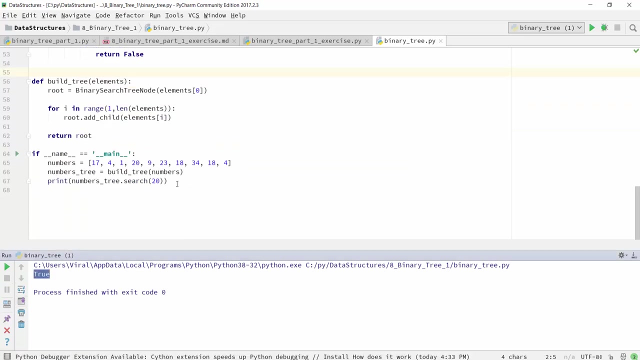 how this looks. so i did this traversal. now i will do this. so numbers tree here: numbers tree dot search. okay, let's search for value 20.. and when i run it, it returns true because value 20 exist in this. now how about 21? when i run it, it will return false because it doesn't exist. 200 also doesn't. 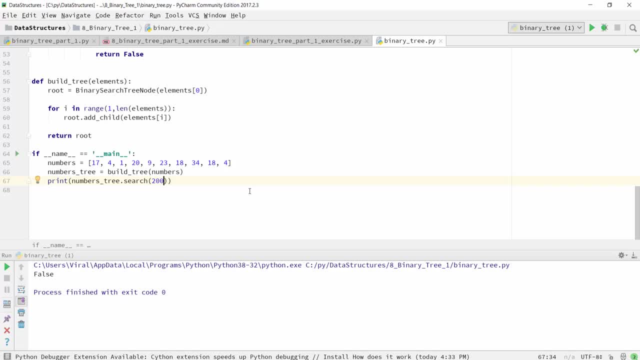 exist. so this makes your search operation very efficient. you achieve order of log and search complexity, which is pretty good. here i'm showing you example of binary search tree which contains string. okay, so it's not just for numbers, you can also use a string as an elements. and here i have all these elements here and i'm checking if uk is in the list and if 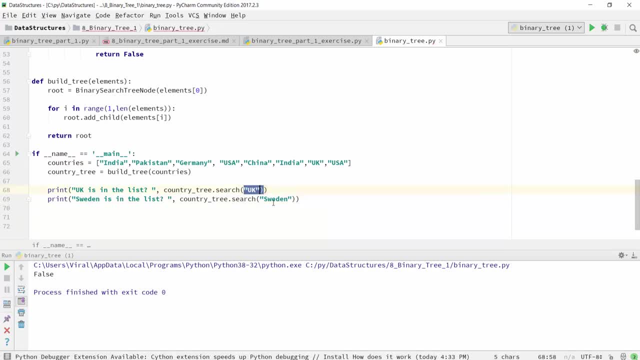 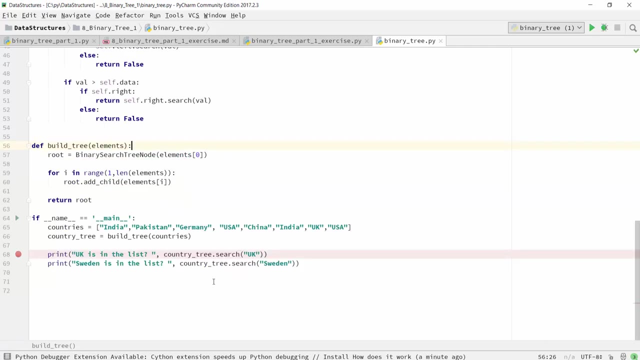 sweden is in the list, okay. so here you clearly know uk is where is uk. yeah, uk is here sweden, sweden, there is no sweden. okay, so let's run this code and see what happens. so here say: uk is in the list, none- okay, so it looks like we get none, because here we need to return this. so this: 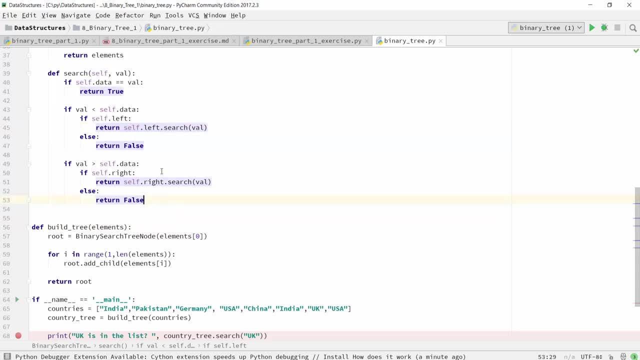 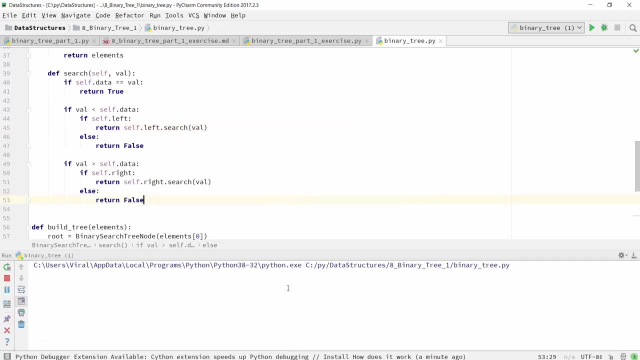 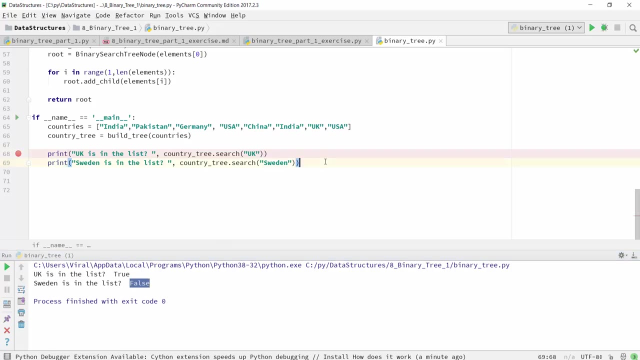 is what i was missing. we need to return, uh, this particular value. okay, so that return was missing and that is the reason we saw none. so let's run this again and here it is saying: you is in the list. true, sweden is in the list. false, if you want to print this particular tree in a 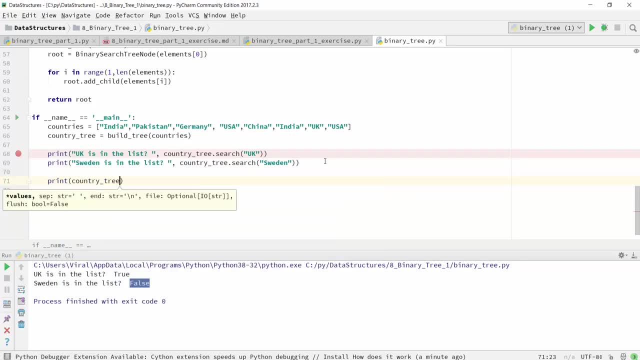 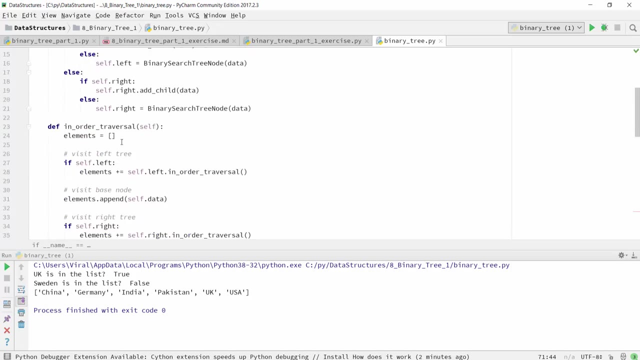 sorted order. you can say country tree dot in order, traversal, run it and you just sorted your countries by alphabetical order. in python you can do less than greater than type of operation with string string as well. well, and that is the reason you are seeing this countries list in a sorted order. 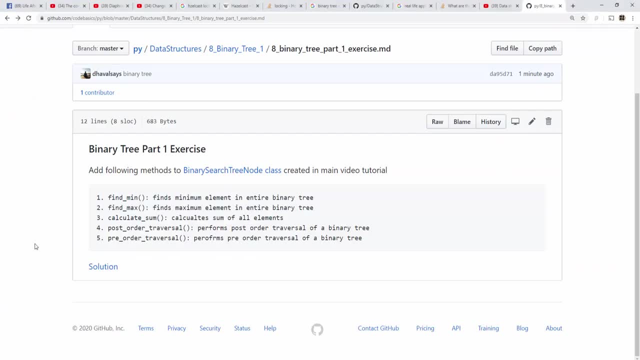 that's all i had for this tutorial. now, the most interesting part of this video tutorial, which is an exercise. i have this exercise for you. what you need to do here is the binary search tree node class that i implemented in this video tutorial. if you right click on this, this is available here. you can see that the whole class is available you. 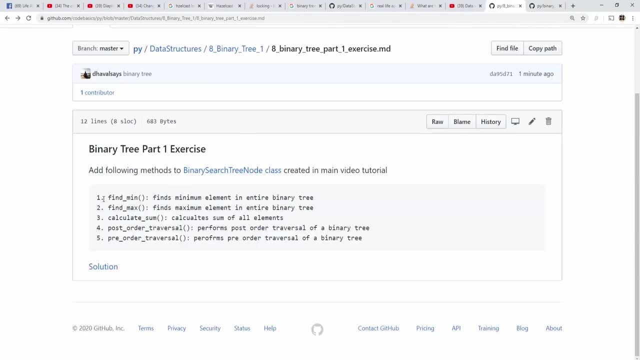 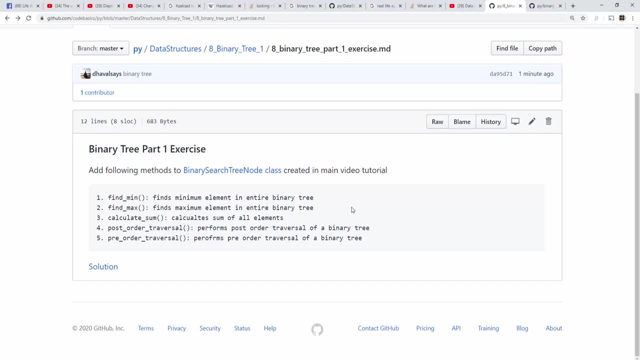 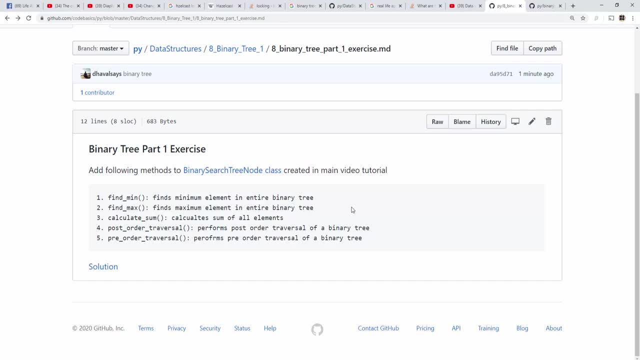